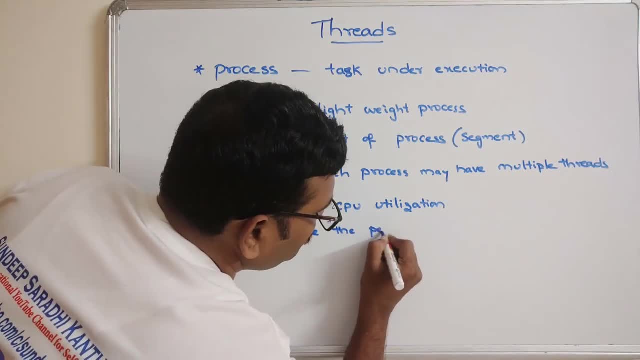 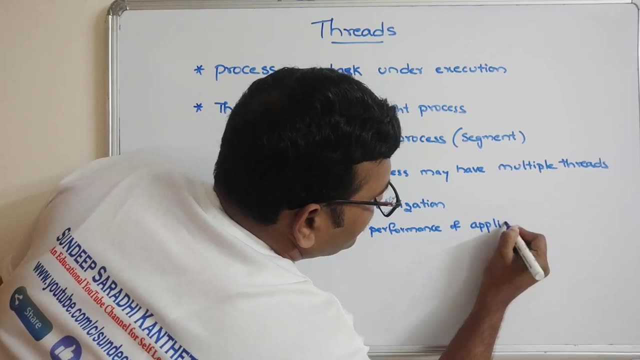 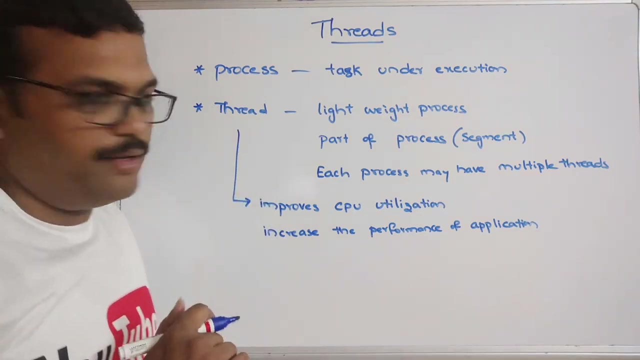 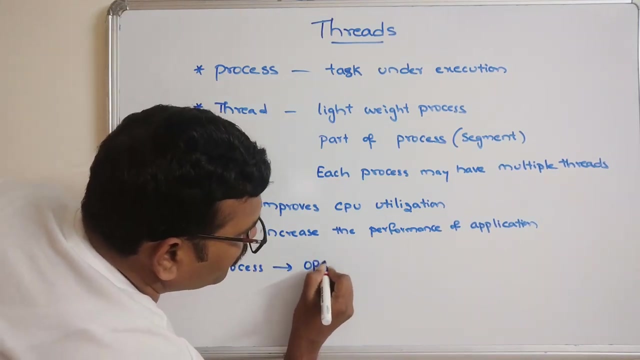 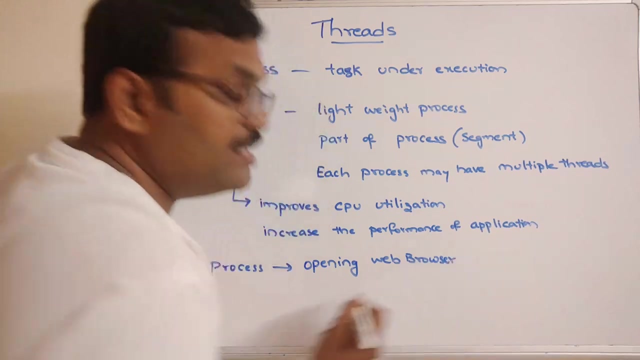 the performance of application. See, I will tell you the example of a process and threads so that you will be understanding clearly. So process means opening a web browser. So opening web browser is a process. So we know web browser, which 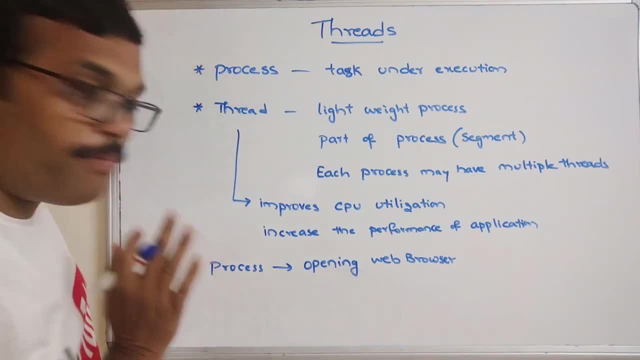 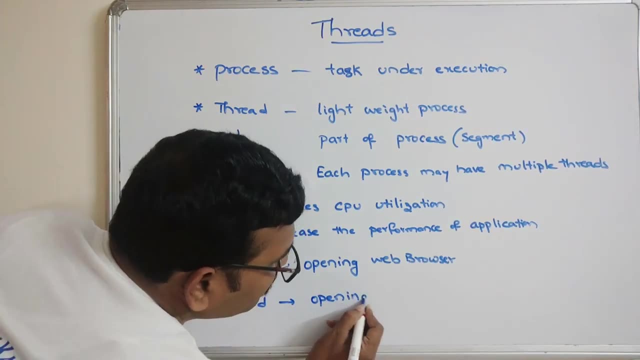 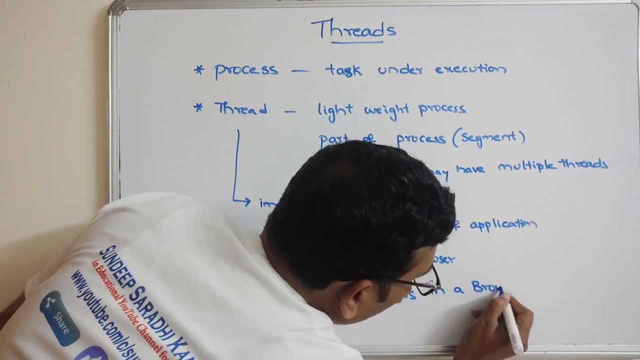 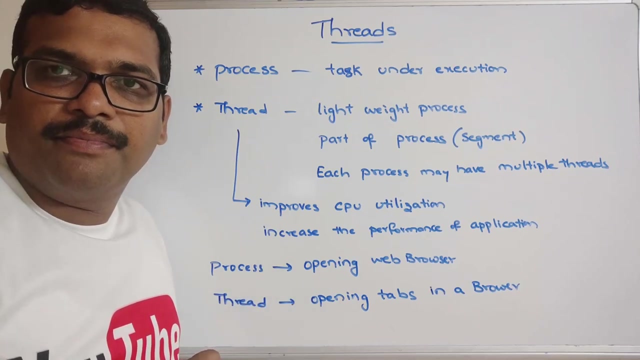 will connect us to the internet. So that is called a process And thread for this process: opening tabs, multiple tabs in a browser. So in a browser we can open a multiple tabs, Right, So that we call it as a thread. 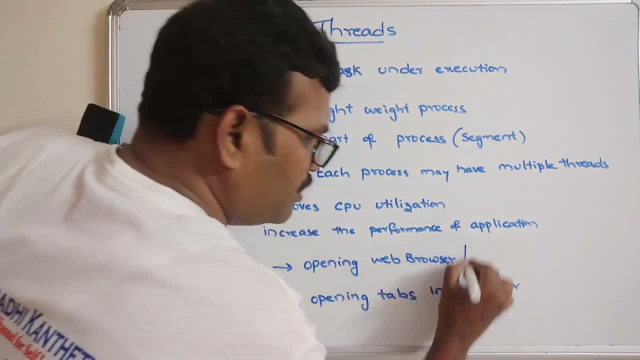 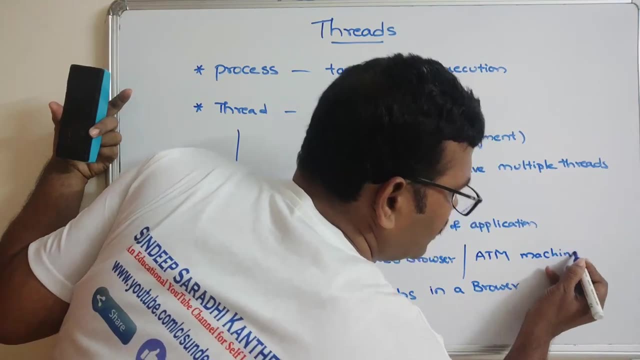 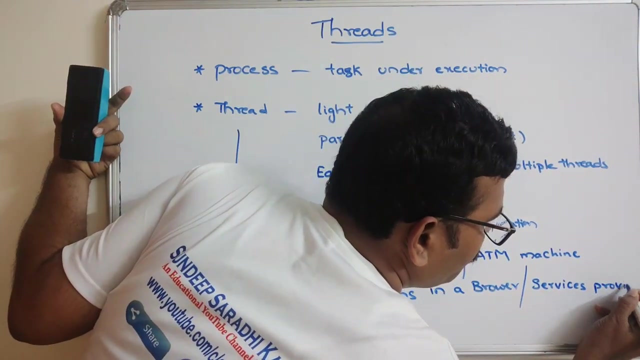 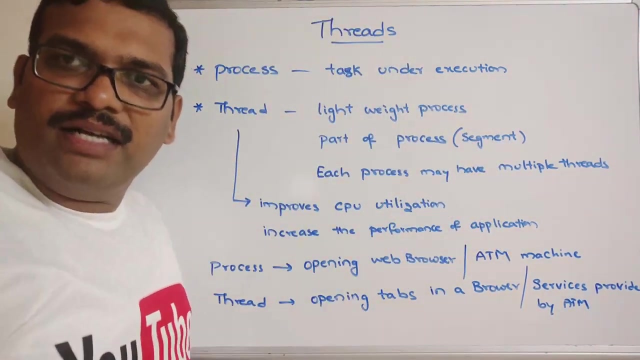 Right. Similarly, you can also say one more example. So ATM machine. consider ATM machine as one process and the services, whatever the services provided by ATM can be considered as threads. be considered as a threads. that means so withdrawal service and mini statement and even deposit, if 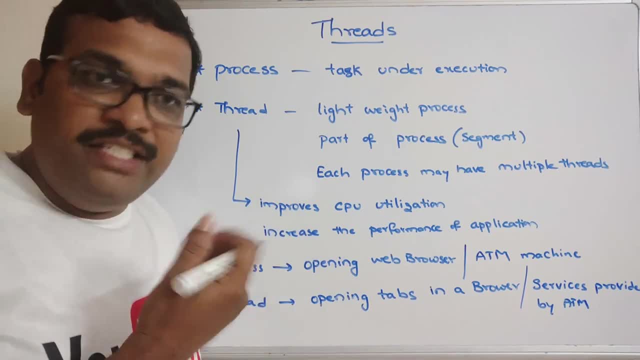 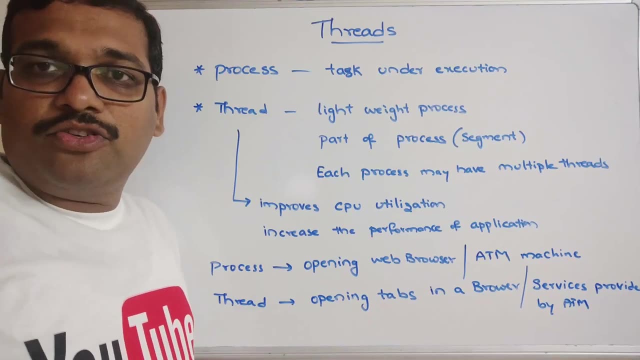 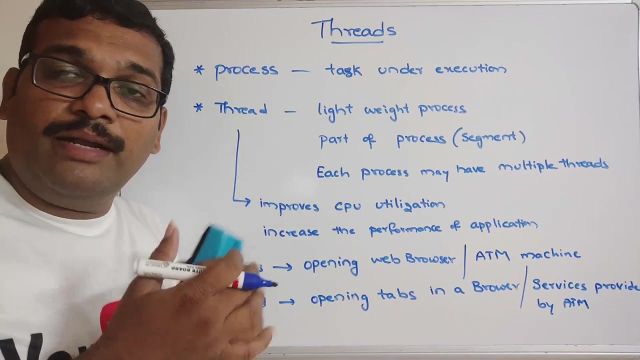 you are going with the deposit machines: deposit right, pin change. okay, mini statement: all these will can be considered as a threads. that means a part of a process, so a process can be divided into a multiple threads. okay, depends upon the application, so it may have a multiple threads. 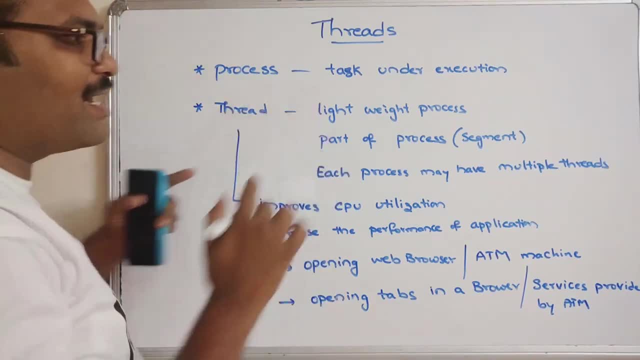 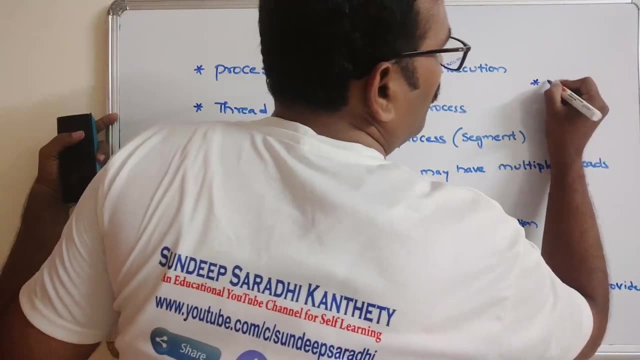 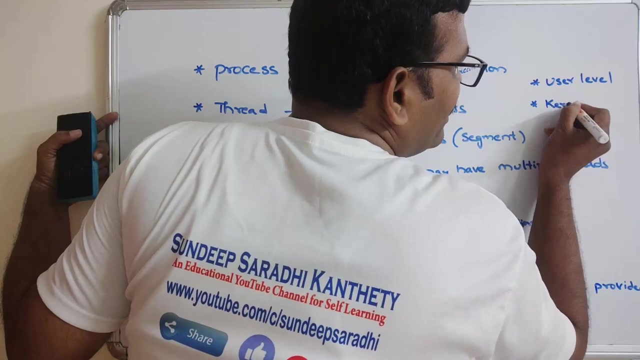 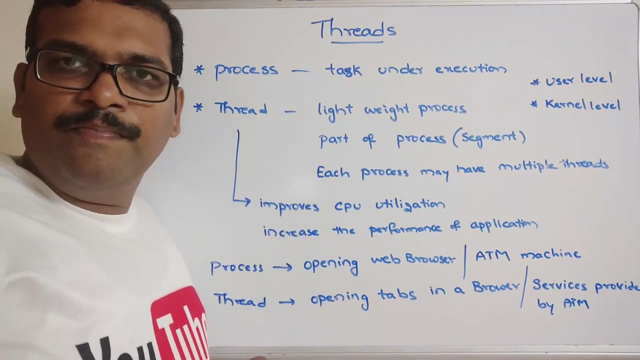 or a single thread, right. and these threads are classified into two categories. so one is user level threads and another one is kernel level threads. kernel level threads: so user level threads will be created by the users and the kernel level threads will be created by using the operating. 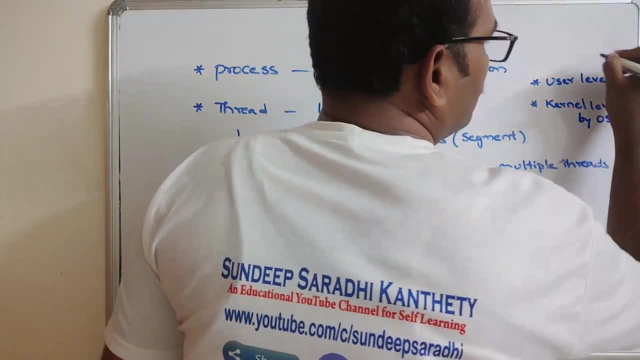 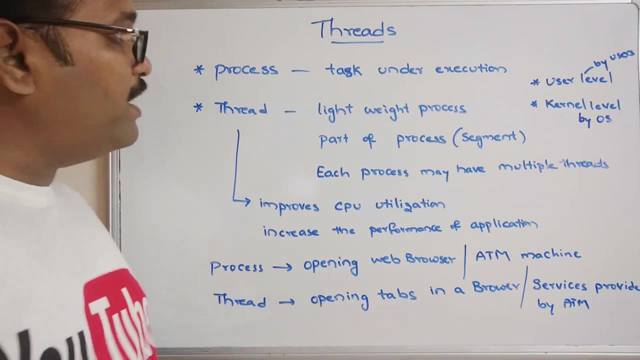 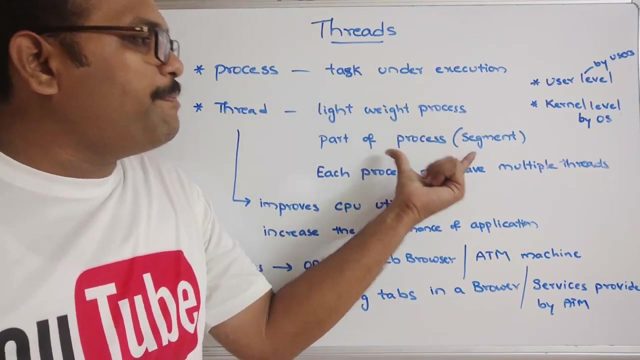 system, right so? which will be done by operating system, which will be done by users, users, right? so that's why we call it as a process is a task under the execution and a thread is a lightweight process. okay, and it's a part of a process or a segment of a process, and each process may have a multiple 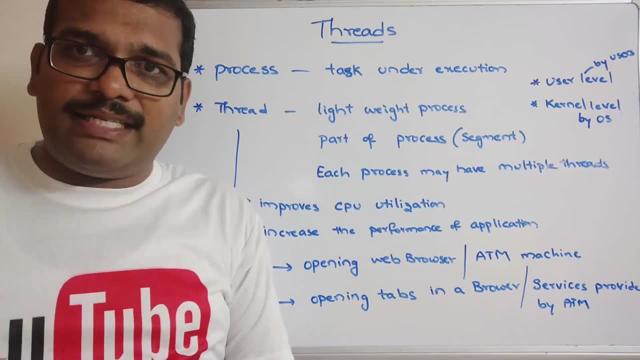 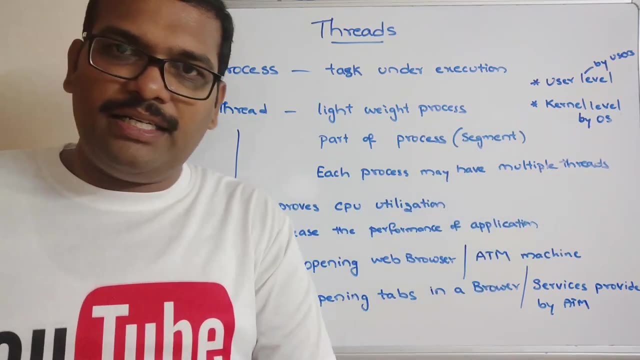 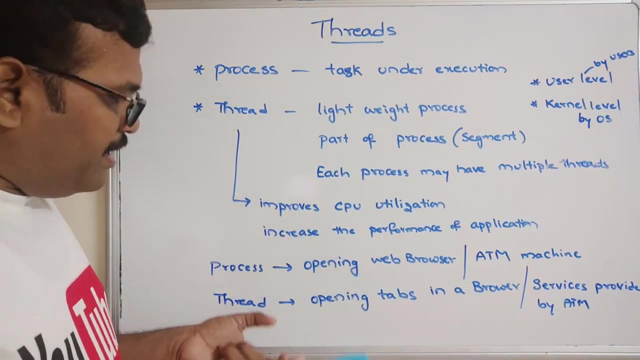 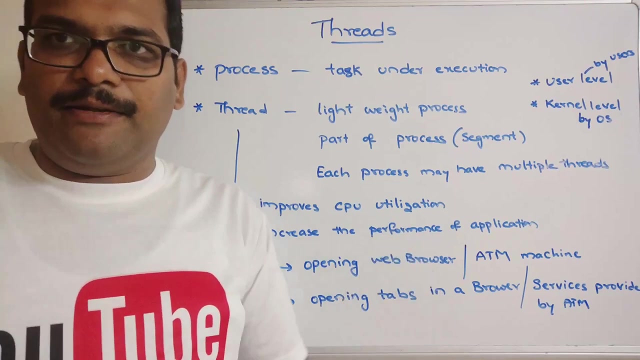 threads, so execution of multiple threads. running of multiple threads is called as a multi-thread, right, so which process will be? having multiple threads and running these multiple threads concurrently is called multi-threading, and running a different process simultaneously or continuously is called as a multi-tasking. okay, multi-tasking and multi-threading. multi-tasking means executing. 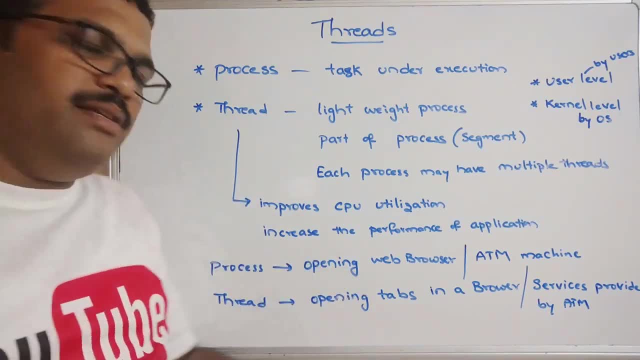 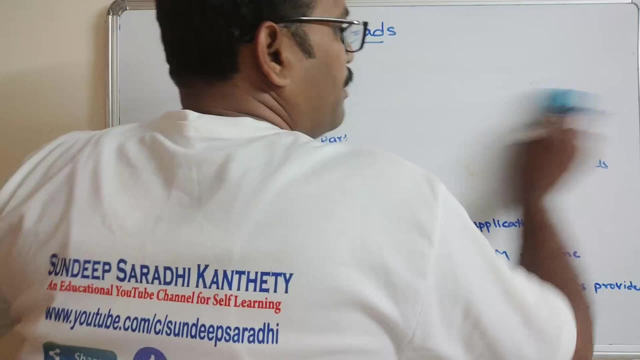 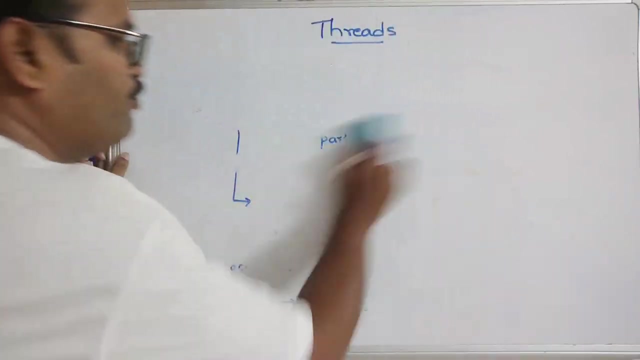 more than one task at a time, and multi-threading means executing more than one thread at a time. right, see, i'll write here and we'll go with a diagrammatic representation. so if you have any doubts, definitely those doubts will be get clarified once you see the image. okay, once you see the image, it will. 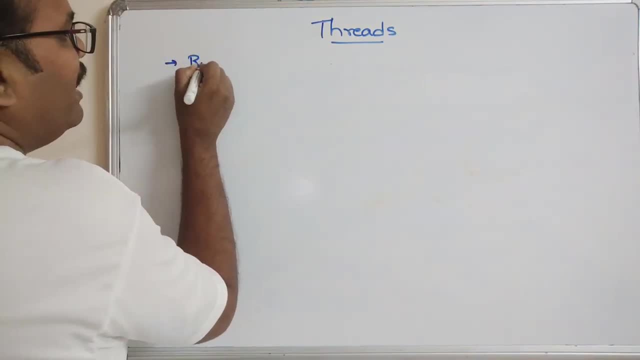 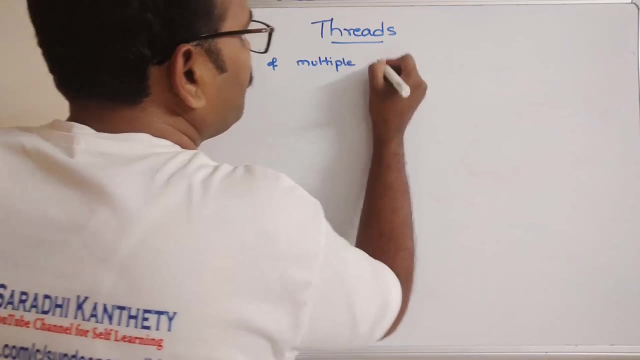 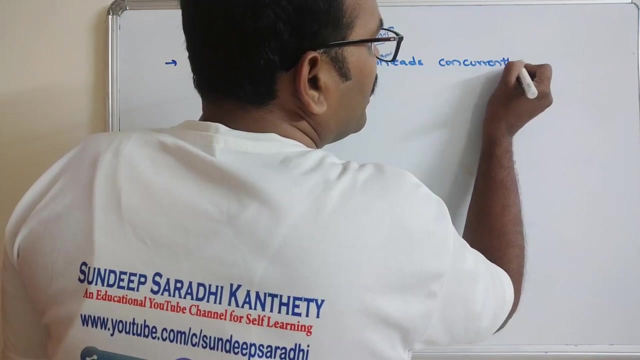 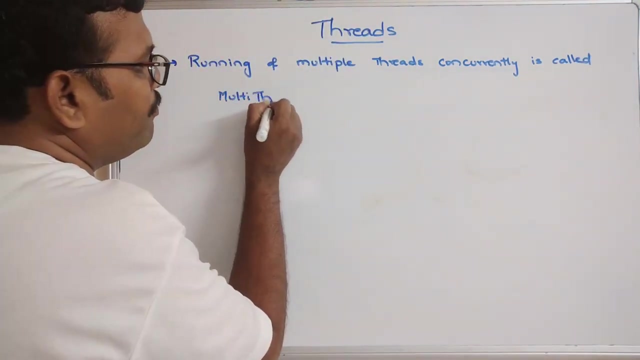 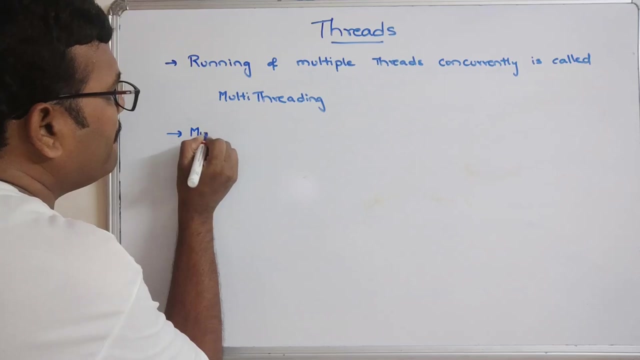 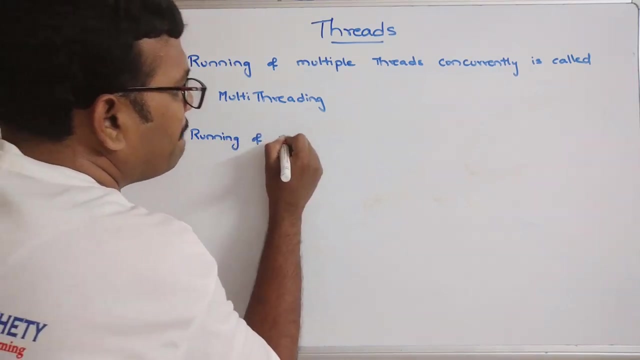 be clarified. so running of multiple threads concurrently- concurrently is called multi-threading. multi-threading: so running multiple threads at a time and running off multiple tasks. the task is nothing but a process, right? so if there is a multi-tasking, then what we are going to do is we are going to run it like this, okay. 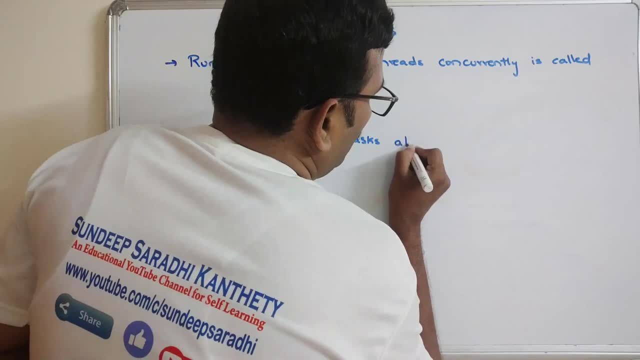 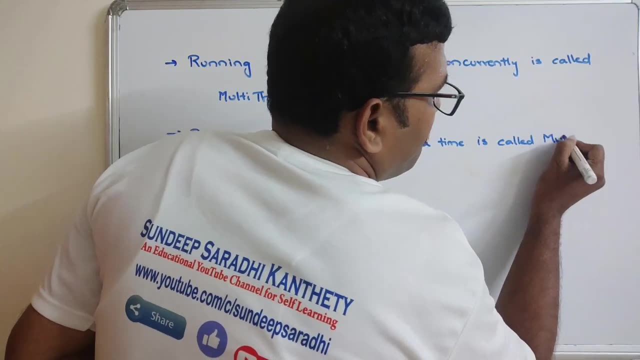 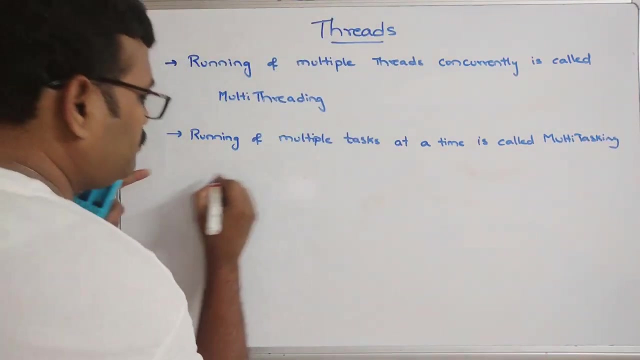 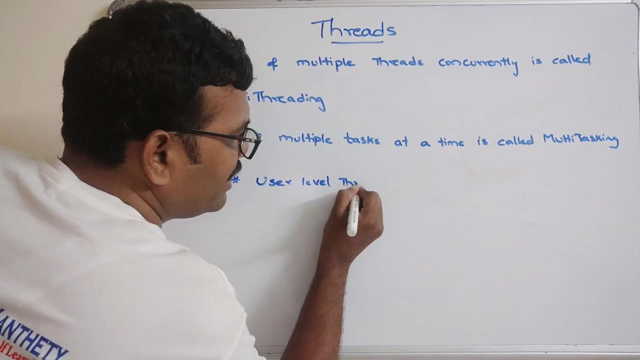 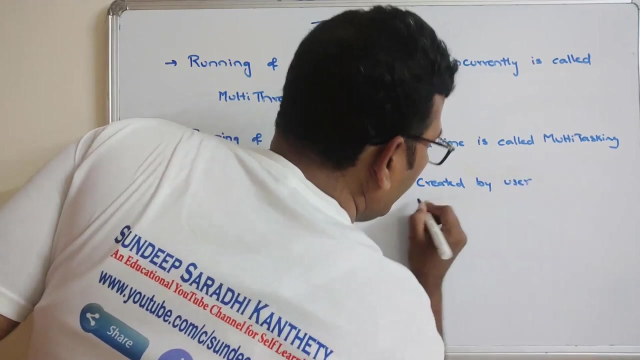 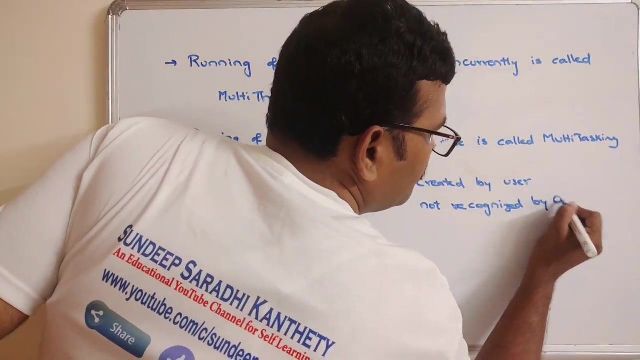 running of multiple tasks at a time is called multi tasking. it's called a multi tasking, right. see. so one. one type of thread is a user level thread. user level thread and created by user and not recognized. it is not recognized by the operating system. it will be recognized only by the user itself. and these are 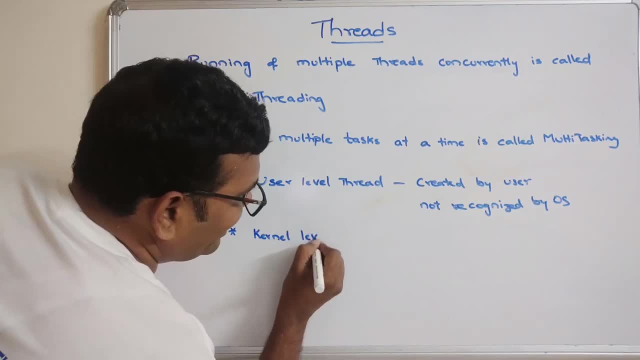 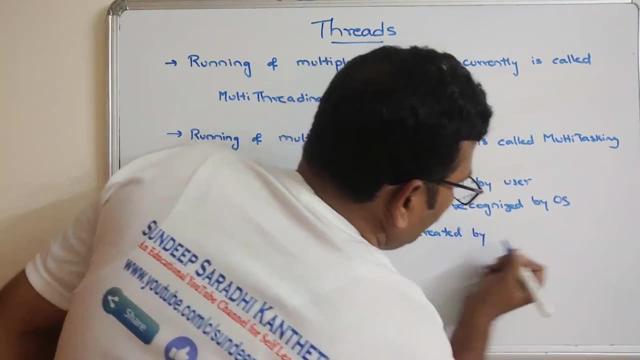 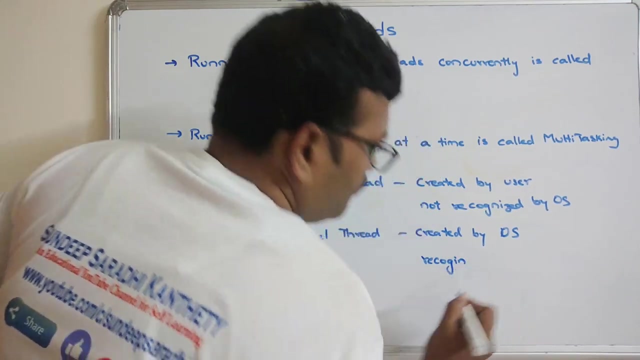 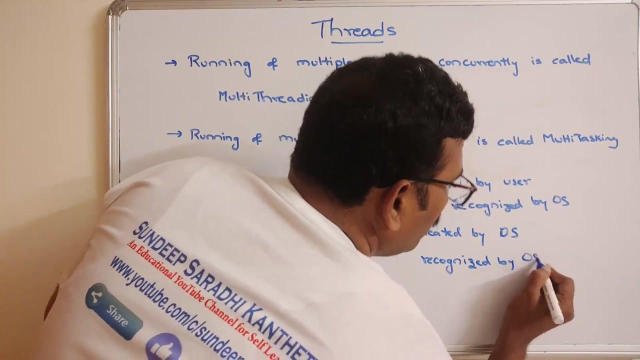 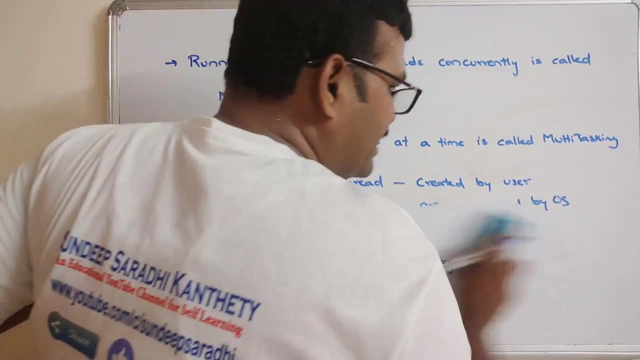 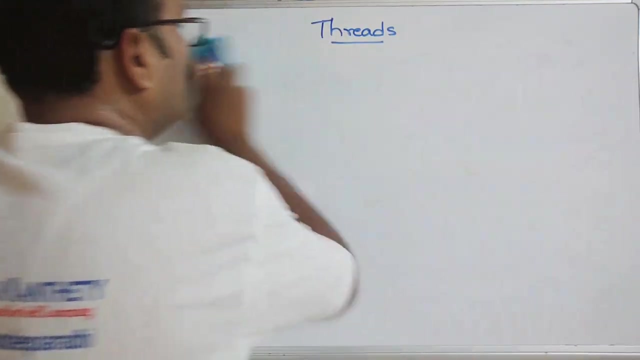 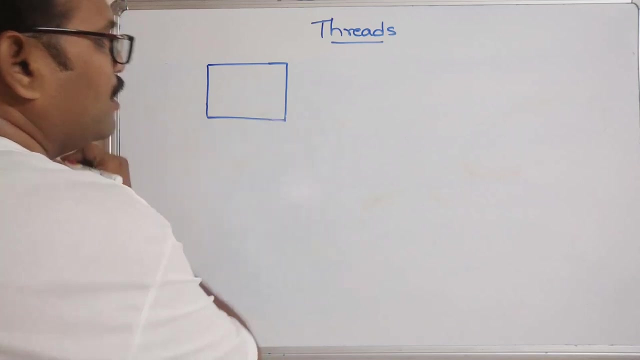 the kernel level threads. the second part is a kernel level threads created by OS, and these are recognized, recognized by our right. so these are the two categories of threads. now we'll see what exactly the proper process looks and how exactly the thread looks see. so let it be, this is a process. this is a process and you can see. 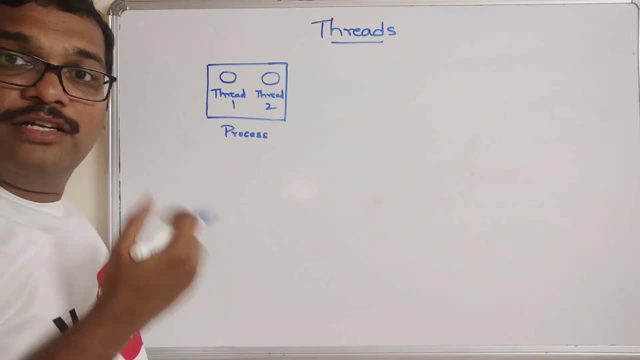 example, let us say this is the threads, so a combination of threads is known as a process. so let us say this is a process, so a combination of threads is a process. okay, process can be divided into multiple threads to run concurrently and to improve the performance and the CPU utilization and 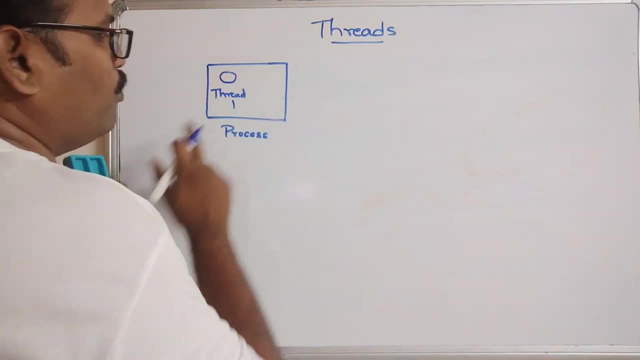 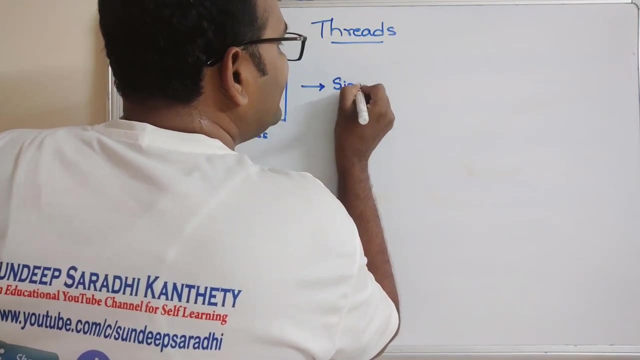 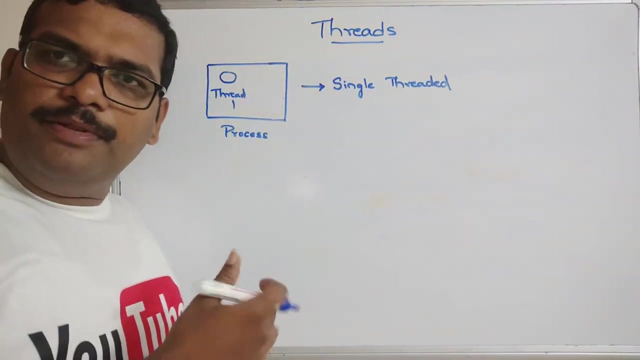 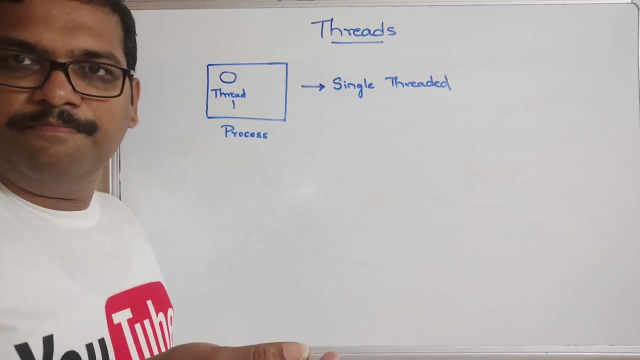 see if the process is having only one thread. if the process is having only one thread, this is known as single threaded process. so it is not mandatory that every process will be having multiple threads, right. so depends upon the application. so the process may have a single thread or a multiple threads, right? so if the 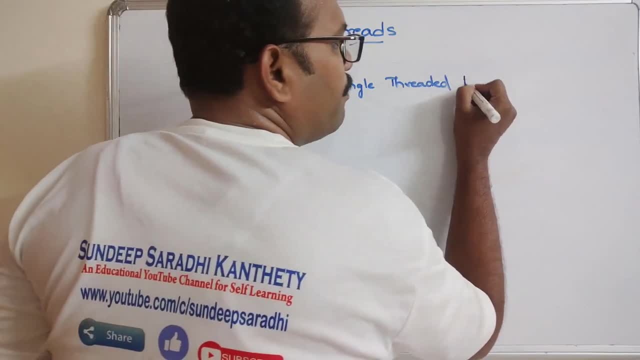 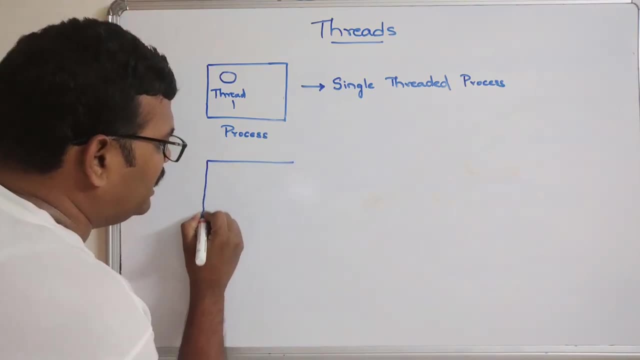 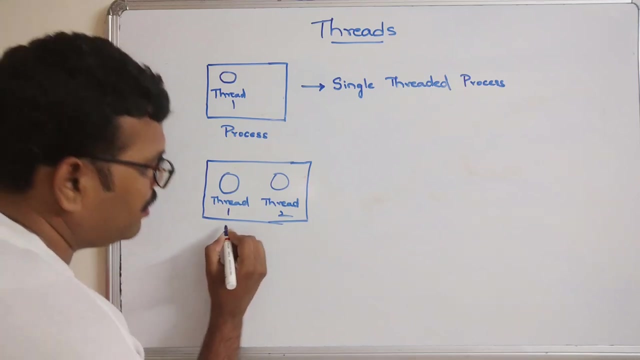 process is having only one thread. that is called a single threaded process. single threaded process: that means only one thread will be there. and if the process is having multiple threads- thread one, thread two- so let it be single thread. so this is a process. so if the process is having a multiple threads, 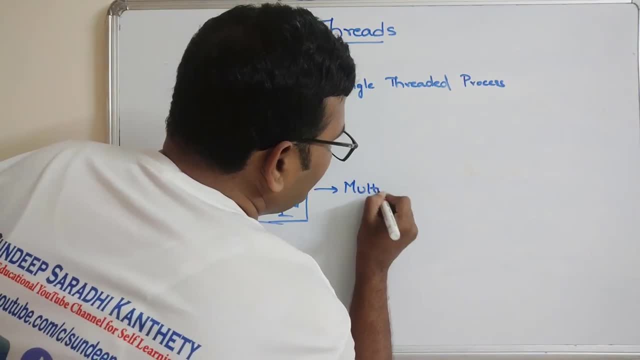 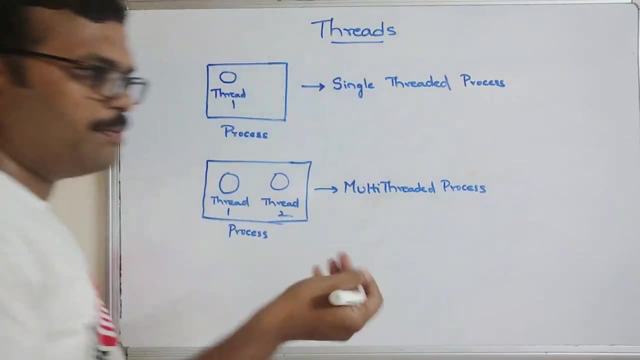 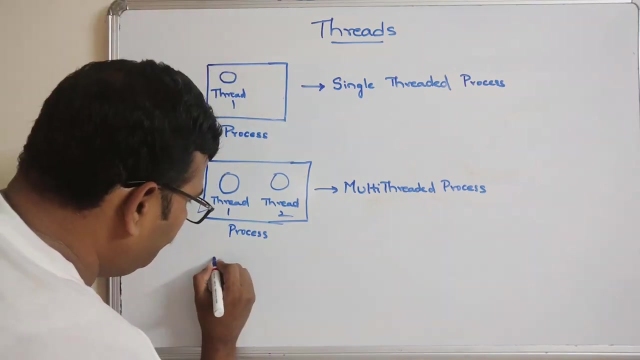 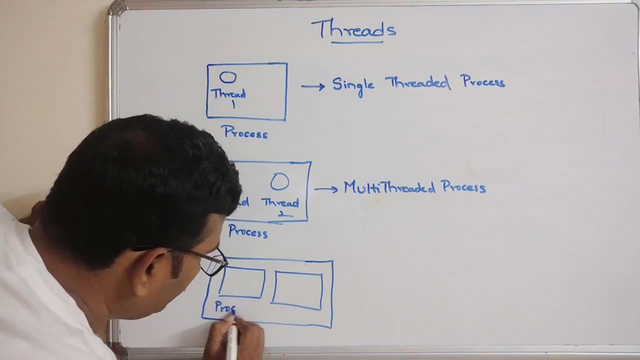 so this is known as Multi-threaded process. the name itself indicates the process will be having multiple threads. multiple threads and there are two more categories. two more categories, So multiple processes. this is process 1 and this is process 2, and here we are having thread 1, and here also we are having thread 1, thread 1.. 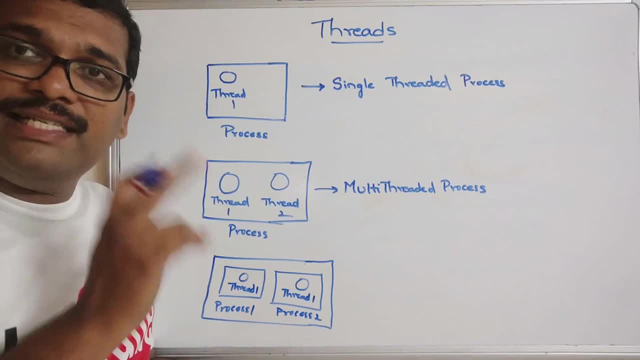 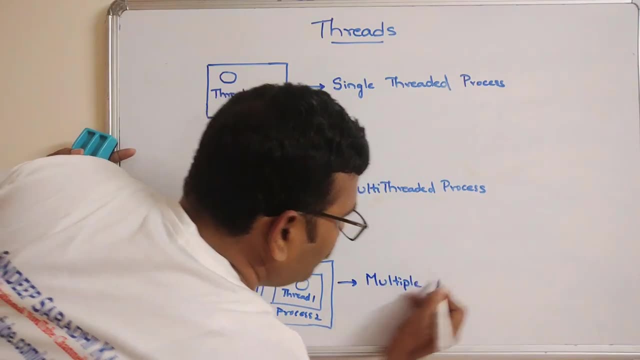 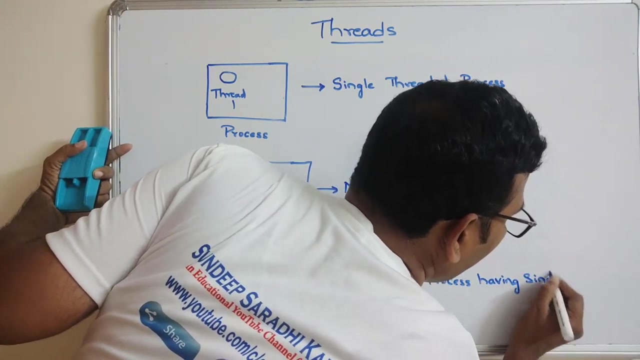 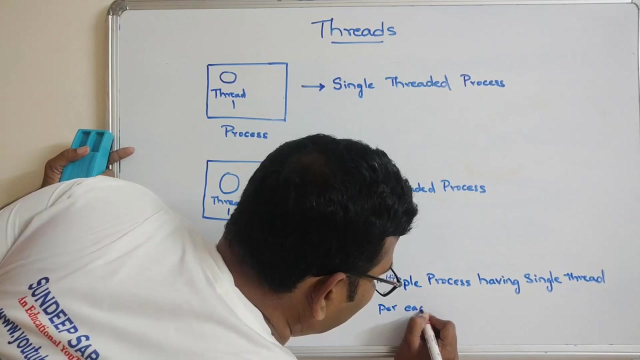 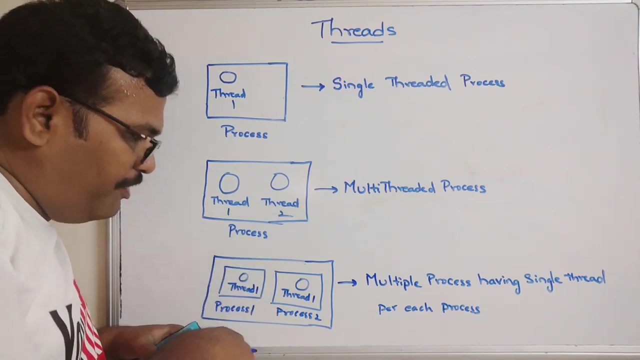 So multiple process having single thread in each process. So this is multiple process having single thread for each process. So there are multiple processes And among these individual processes again we are having only one thread. So this is the third one. 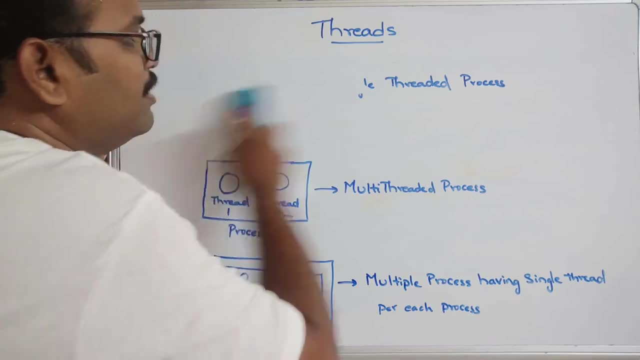 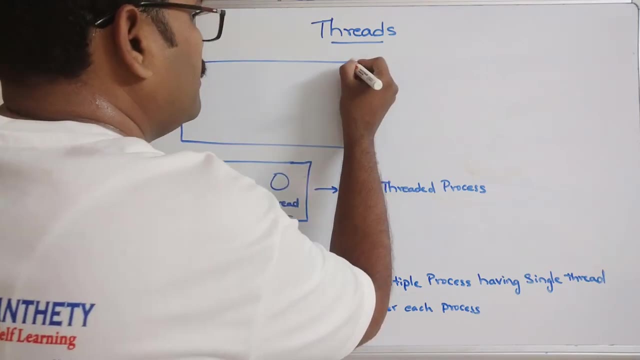 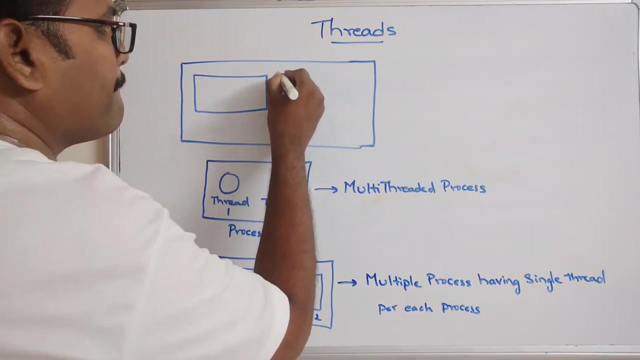 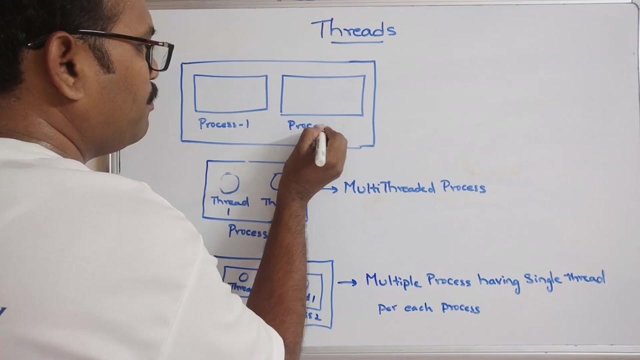 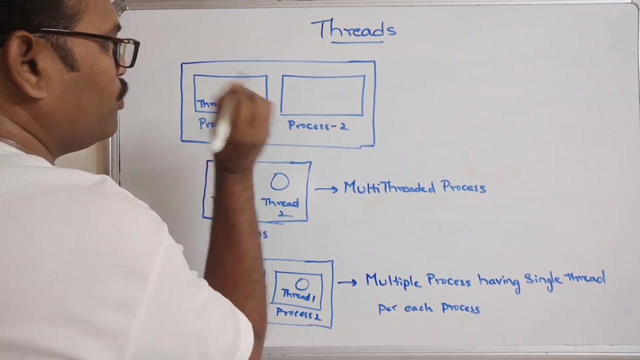 And the next one having a multiple process and in each process we are having multiple threads. Let us take this one. So this is process 1. And this is process 2.. And this is thread 1. And this is thread 2.. 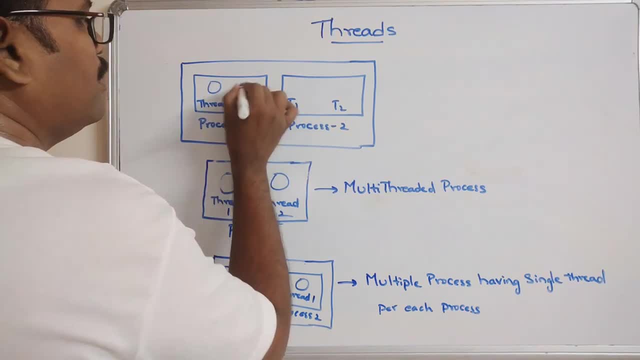 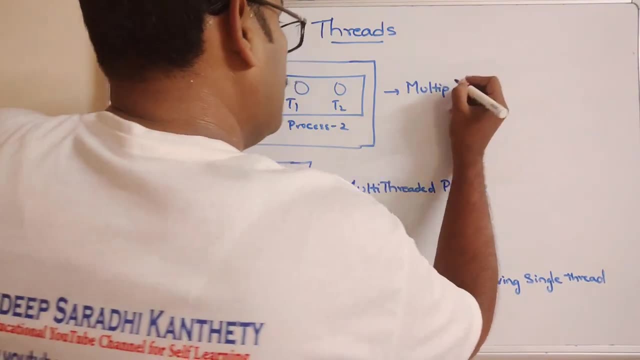 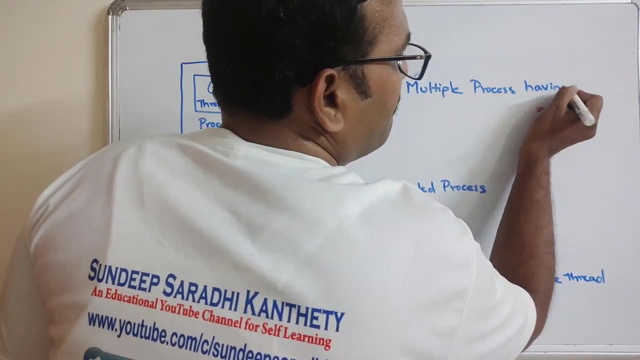 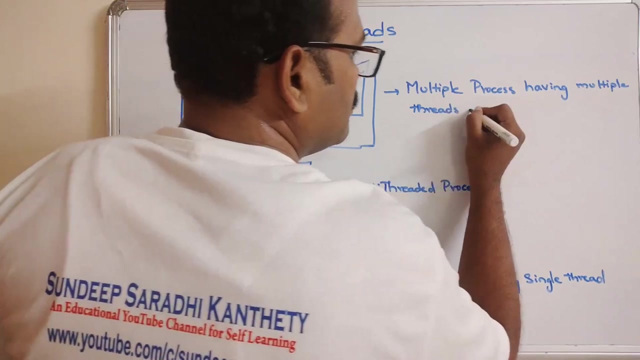 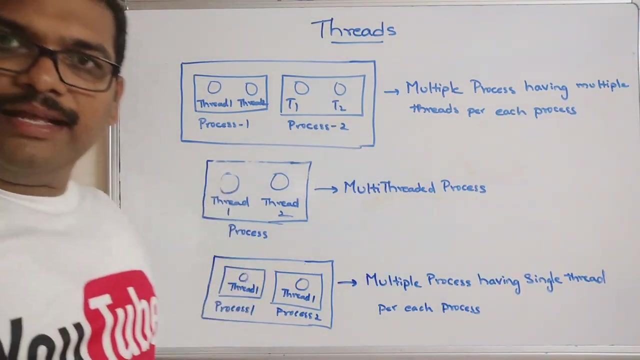 So thread 1, thread 2.. Right, So you can see here: this is multiple process having multiple threads for each process, Each process having multiple threads. So there are four categories. So there are different categories. Okay, 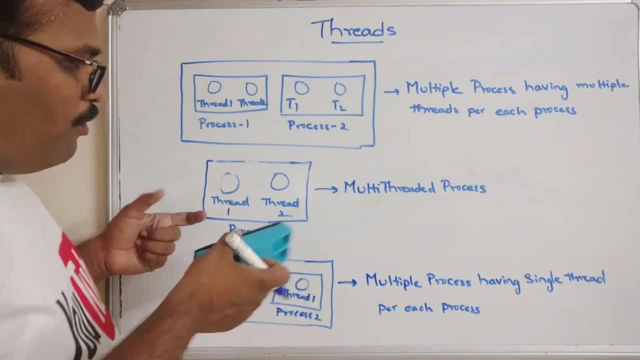 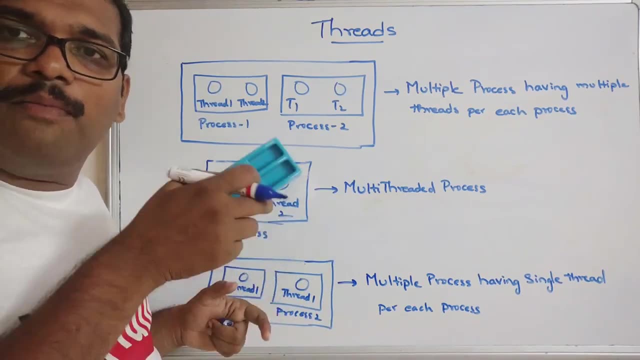 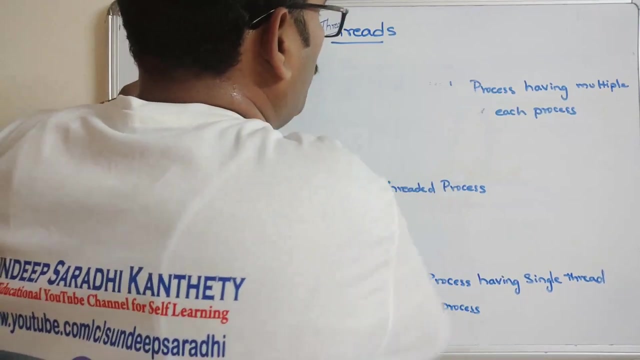 Different categories, And so by creating a multiple threads for a single process, So these threads will share the common memory and the data of that particular process. Right See, I will write down here One important point. So if a process is having multiple threads, 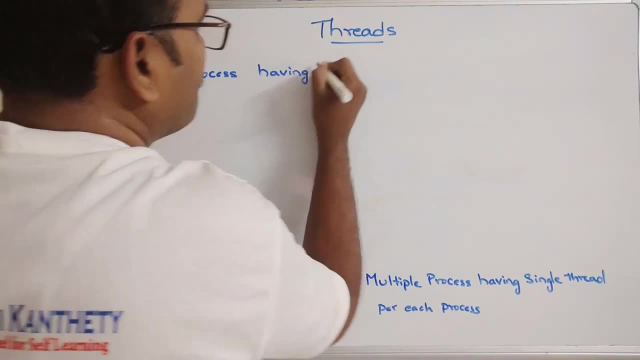 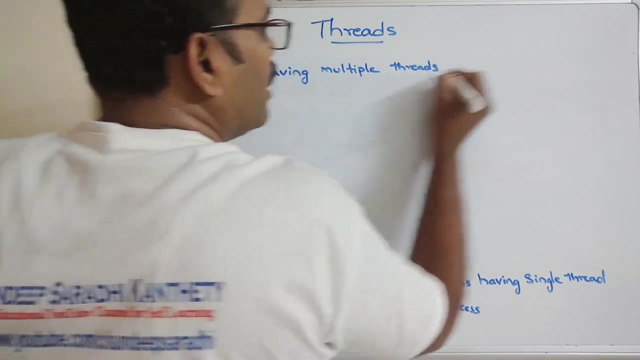 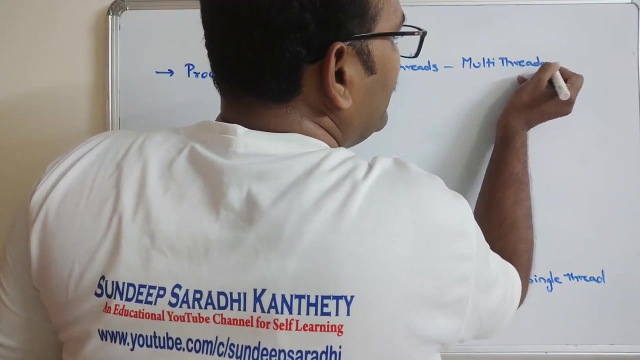 Process, having multiple threads, Right? So what we are telling this one? this is called a multithreaded process. Just now we have discussed it, Right So, multithreaded process. So if the process is having a 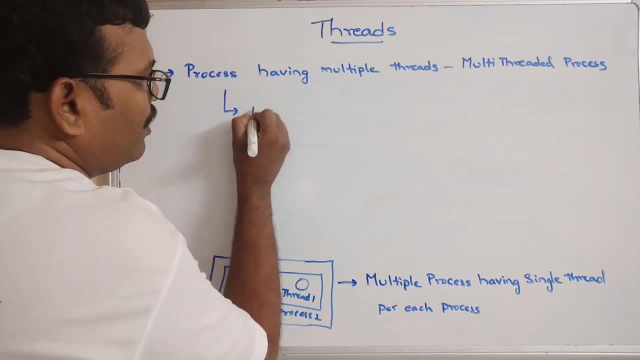 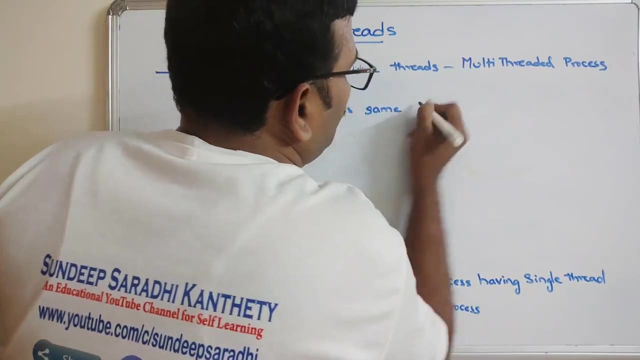 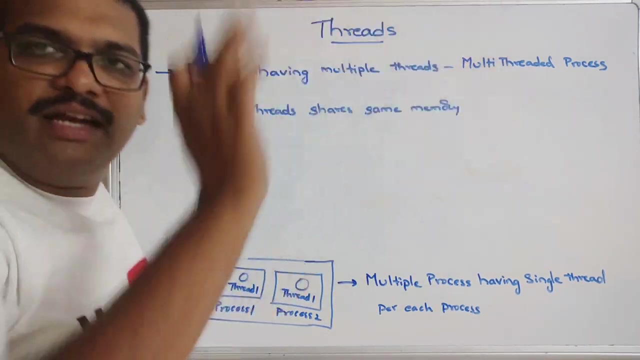 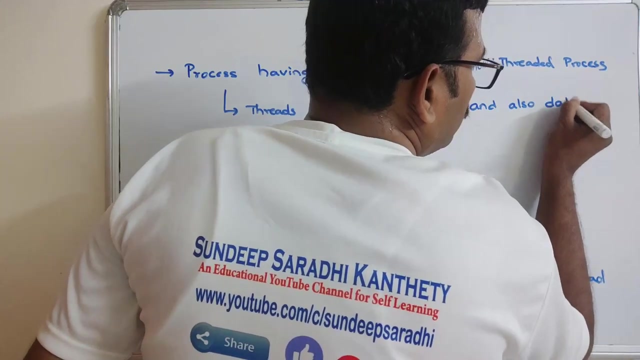 threads, so these threads shares same memory, because so all the threads belongs to the same process. so the memory will be shared among all the different threads. same memory and also data can be shared and also the data will be shared. okay, for example, in previous, just now, we have seen the 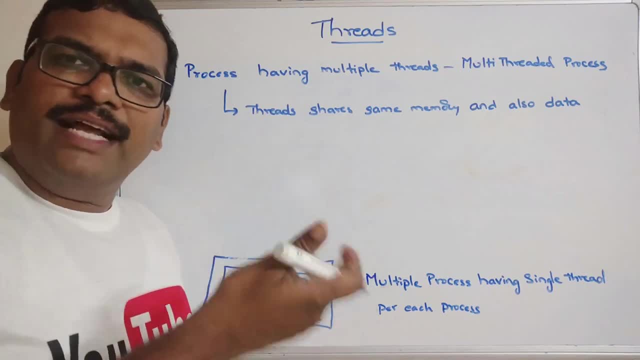 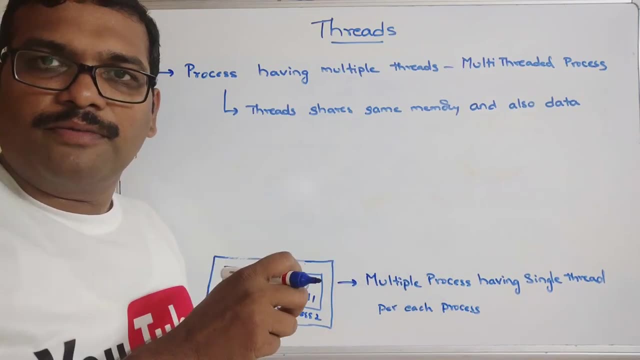 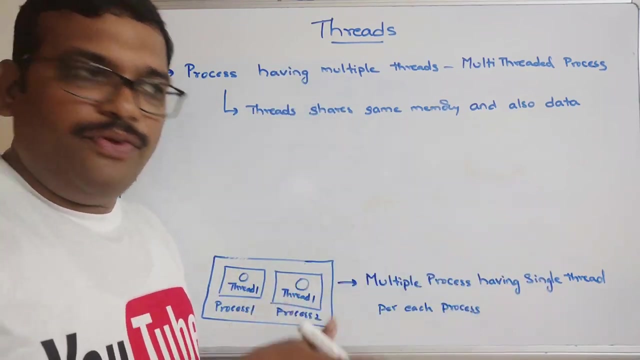 example, that ADM machine is a process, so all the services will be comes under the threads. right, so all the services will be related to the single bank account. okay, so that bank account, the account holder itself, is a one process. so if two persons are having, I mean two persons are there, so one person is having one. 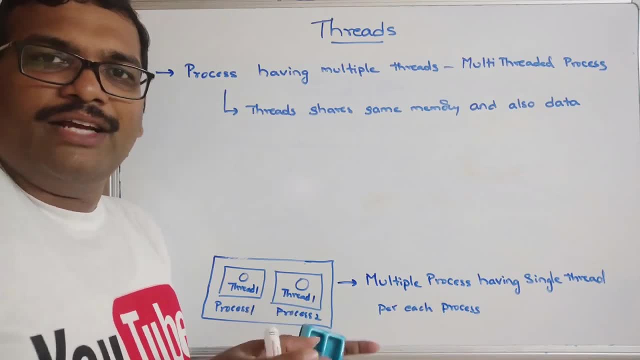 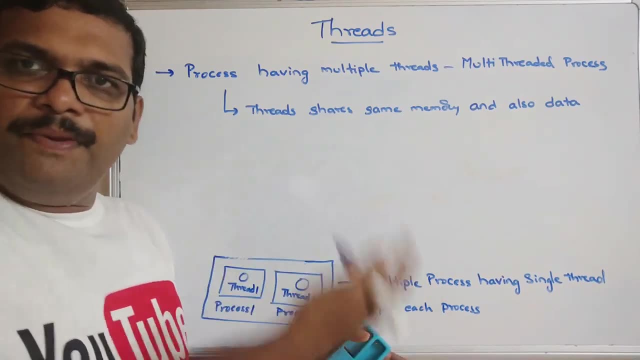 account and another person is having a one account and another person is having a one more account. so these two accounts, we can consider them as a multiple process and each process for each account. we can generate the PIN, we can generate the mini statement. we can avail the service of withdrawal. we can avail 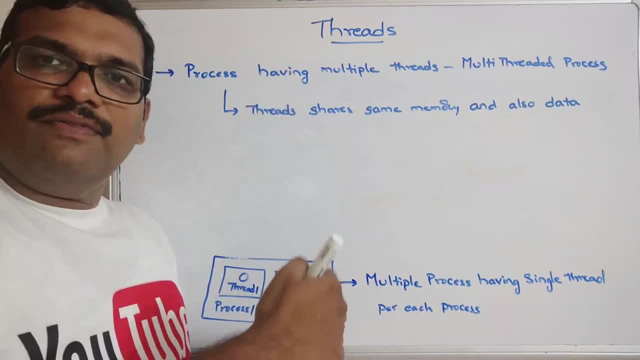 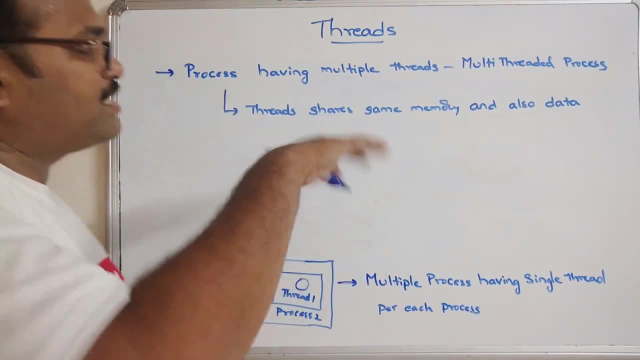 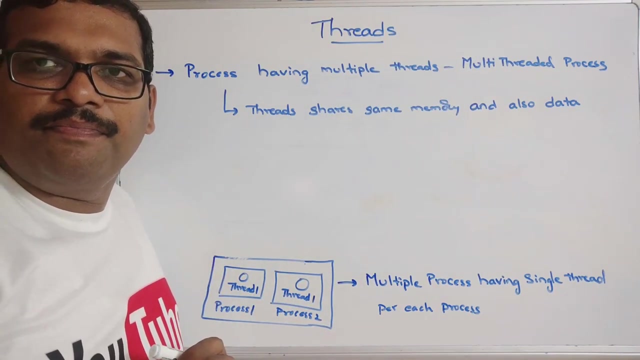 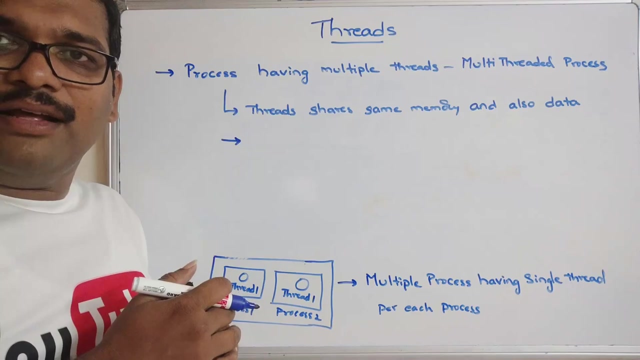 the service of deposit, and also we can use all the services of these ATM for another account also. so such means all the threads of the same process will be sharing the same memory and same data. right and also and also switching between one thread to another thread is. 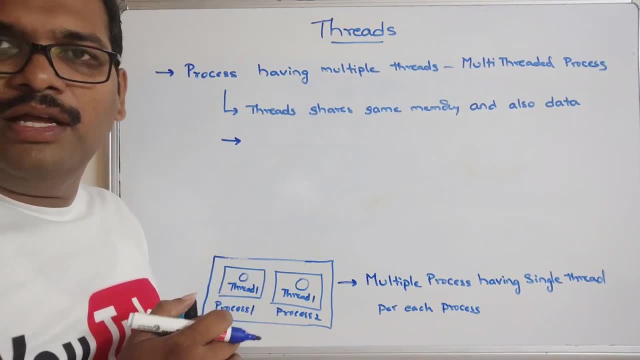 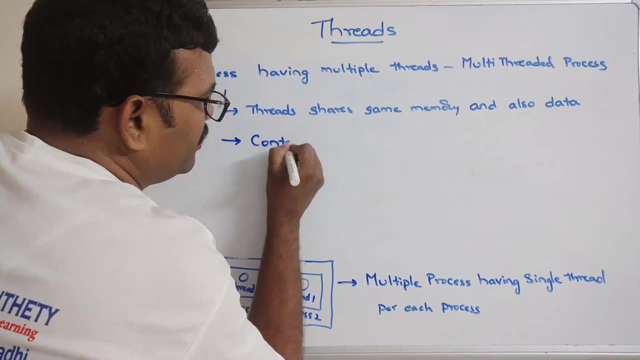 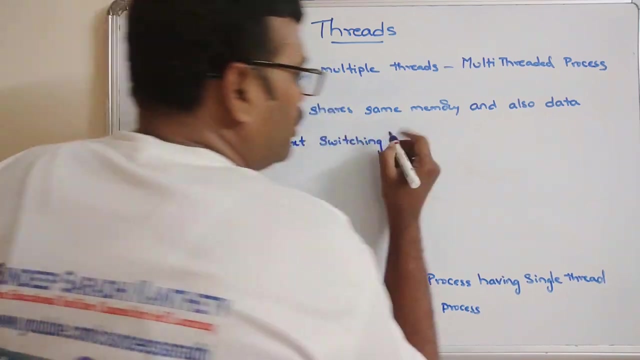 also very simple. okay, so execution of one thread to another thread is also very simple, so that we call it as a context to switching, context switching. so execution, or navigating from one thread to another thread, right context switching- is very simple because both are having in the same memory, both are